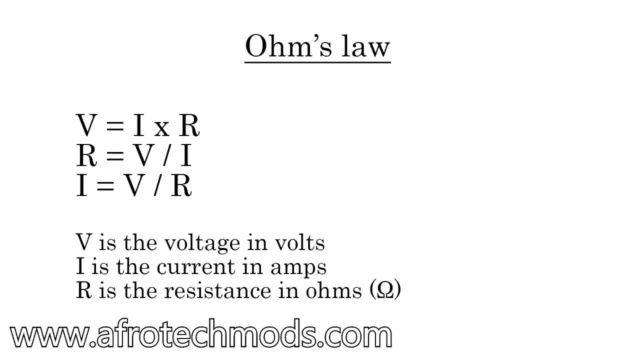 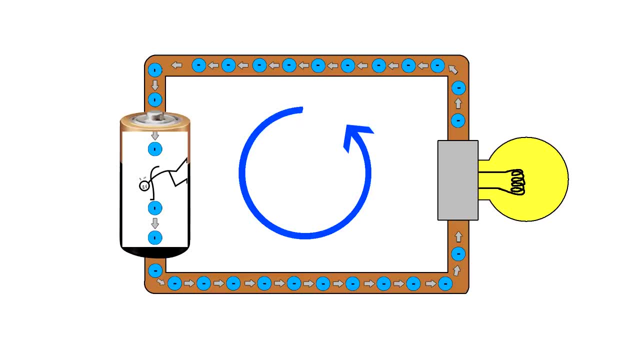 In this video I'm going to talk about electrical resistance, Ohm's law and how to pick a resistor to limit current in an LED circuit. In previous videos I talked about how voltage can behave like a pushing force, pushing electric current around a circuit, But in one example I connected an LED. 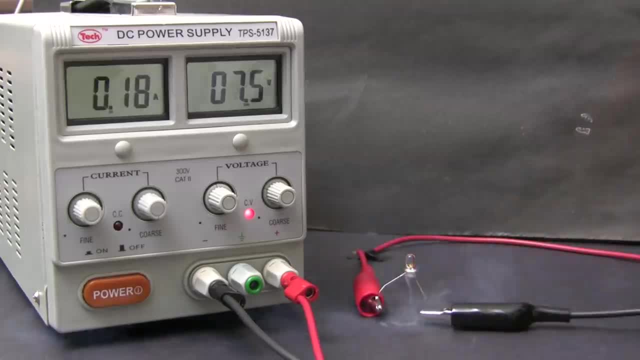 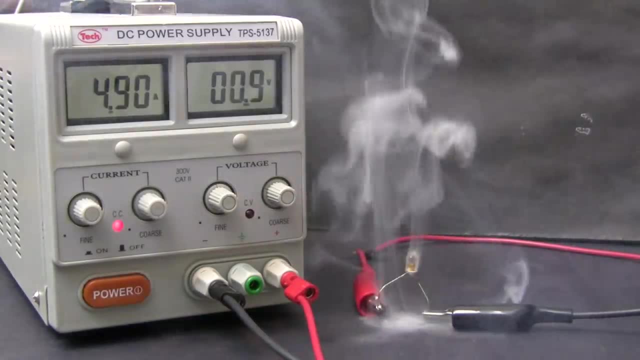 straight to 7.5 volts. way too much current flowed and the LED blew up. So you can see how it would be useful if there was something that could resist the flow of electrical current, something that could tame the flow in a controlled way. That device is called a resistor, and here are some. 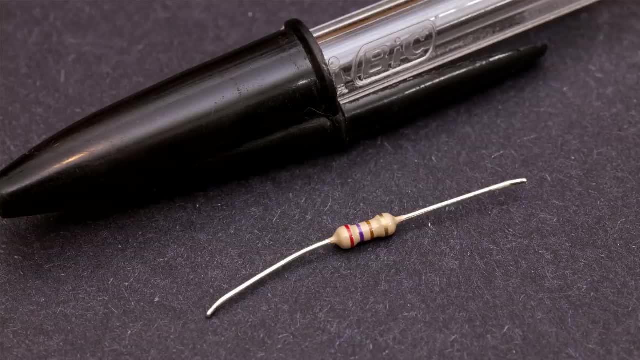 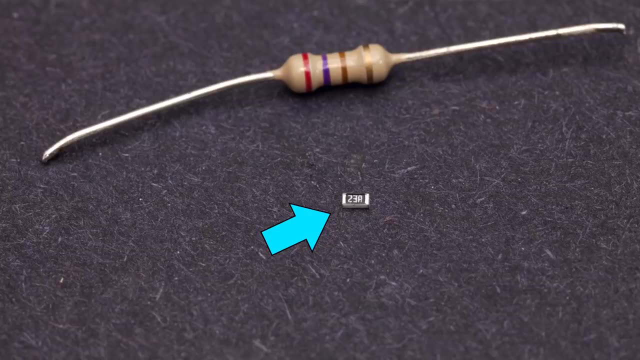 examples of what resistors can look like. We've got a very basic resistor over here, which is the kind of resistor that most hobbyists would use at home when constructing circuits, And over here we have a tiny surface mount resistor. This is something that you'd expect. 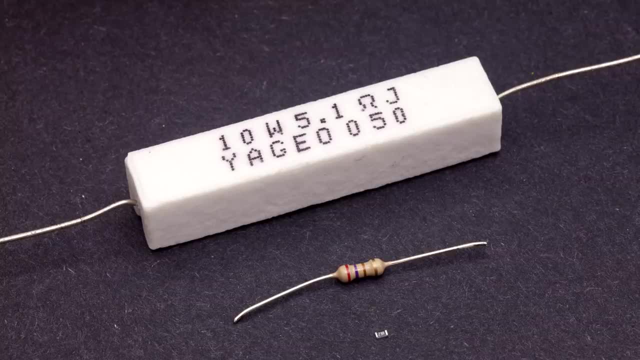 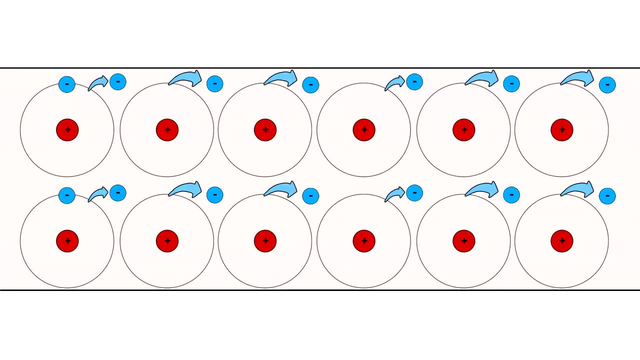 to see in a small device like your phone, And this big resistor is the type of thing that you'd use in a large power supply. So how do these resistors work? Remember how, in my video about current, I talked about electrons jumping from atom to atom all at the same time like a conga line? 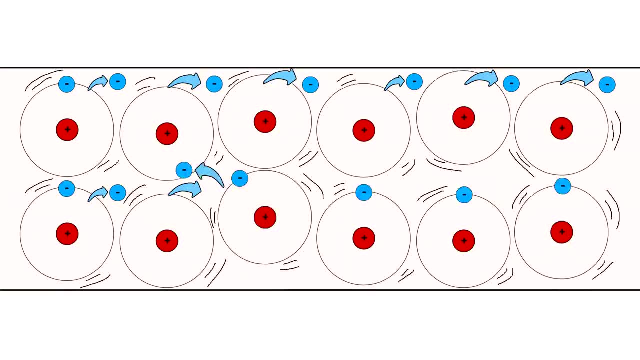 Well, in reality, this process is not 100% efficient. The atoms in a material like copper wire are always vibrating around just a little bit, and this is because of the heat energy that they have. When electrons try to move through the wire, sometimes they'll bump into an atom. 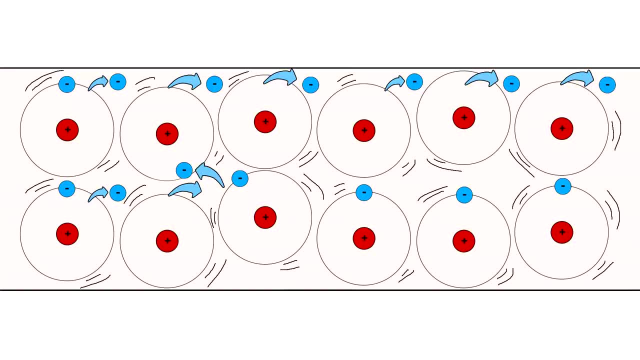 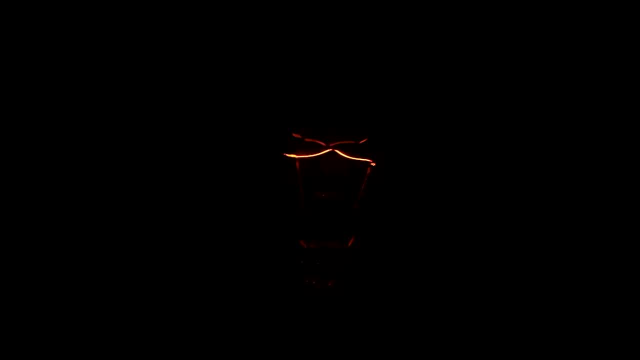 that's in the way and, effectively, the flow of current gets resisted. As this happens, some of the kinetic or movement energy from the electrons gets converted into heat, And this is a fundamental principle behind how electric heaters and incandescent light bulbs work. 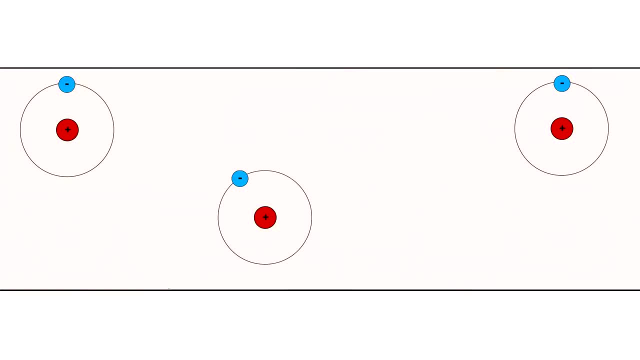 But it's not just metals that have the property of resistance. Resistance can exist simply from the fact that some materials just don't have a suitable arrangement of atoms for electrons to flow through, and some materials just don't have enough free electrons floating around for large. 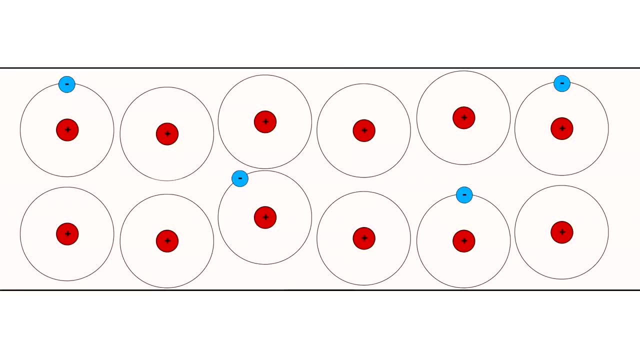 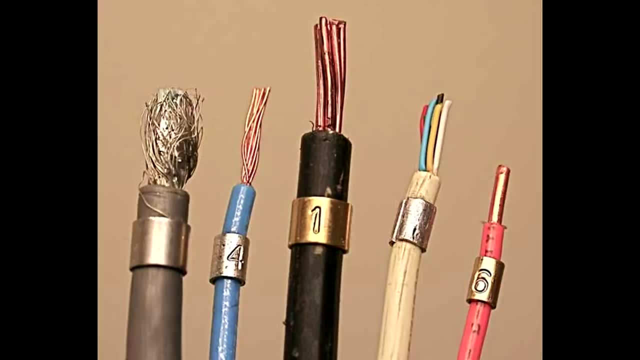 amounts of current to flow. Keep in mind this is a huge simplification and this is not how actual atoms and electrons are going to look and behave at the subatomic level. Nearly everything in the universe is going to have some resistance to electrical current, and metals tend to have. 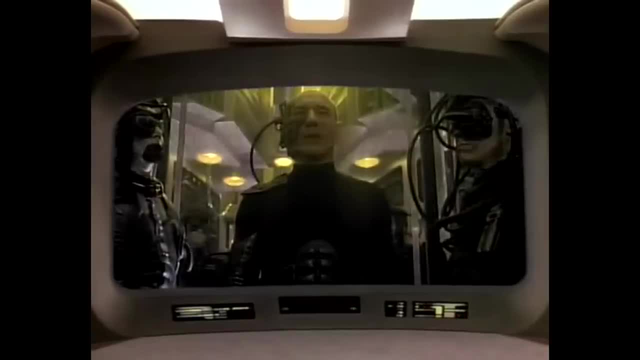 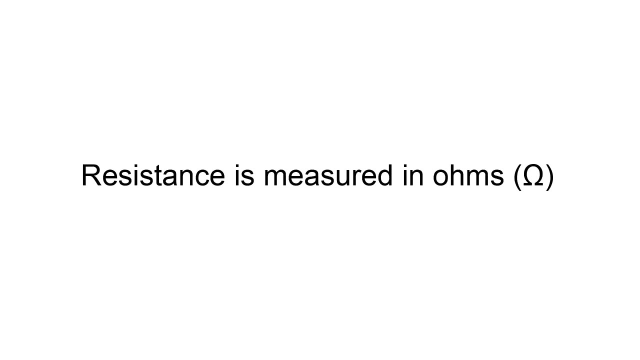 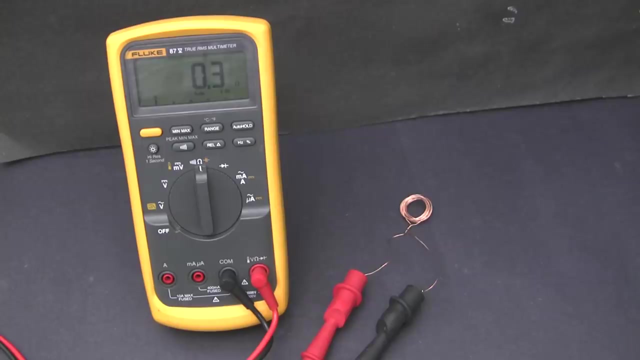 the least resistance. I am Locutus of Borg: Resistance is futile. Sorry, I had to put it in the video somewhere. We measure the amount of resistance with a unit called ohms. The symbol is the Greek letter omega. To give you a sense of scale, a resistance of 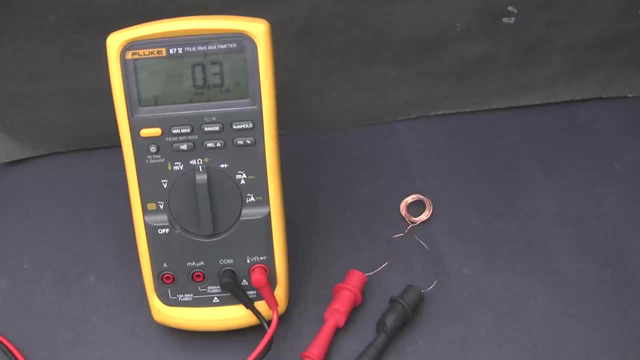 under one ohm is considered to be very low resistance. That's something that you'd expect to see from a bad conductor of electricity like this dried out piece of carrot. This thing that I'm using to measure resistance is called a multimeter, and it can measure the resistance of almost 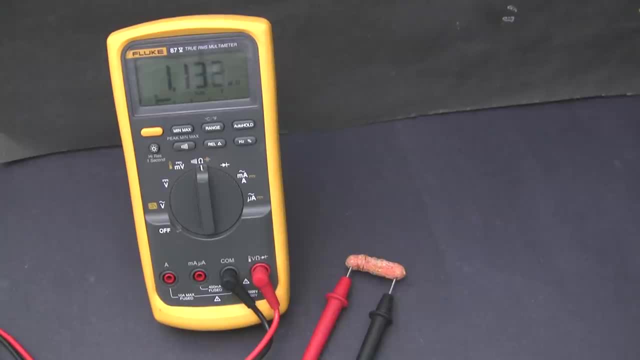 anything. I have a separate tutorial on multimeters, and I recommend you watch it as soon as possible to learn more about this important tool. Now, if you're playing with electronics at home, you'll be using resistors that look like these. I'm going to show you how to measure resistance. 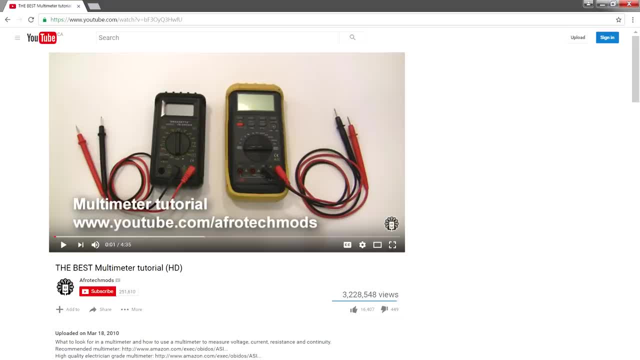 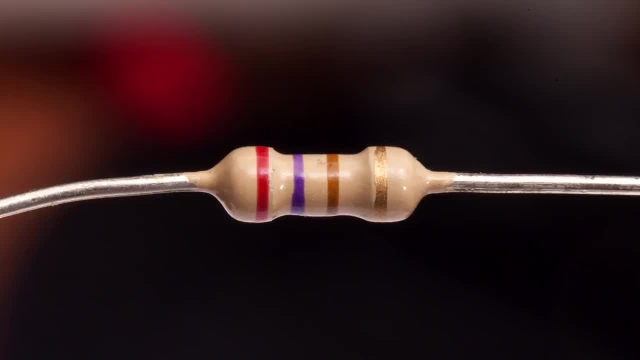 with a multimeter. I'm going to show you how to measure resistance with a multimeter. and I'm going to show you how to measure resistance with a multimeter. If we remove this一次틴, if we add two ohms to it, what happens on the multimeter? 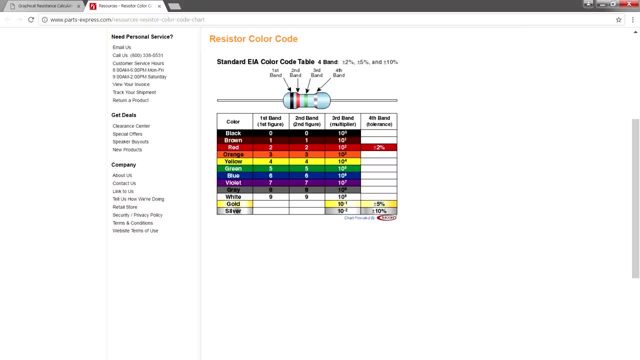 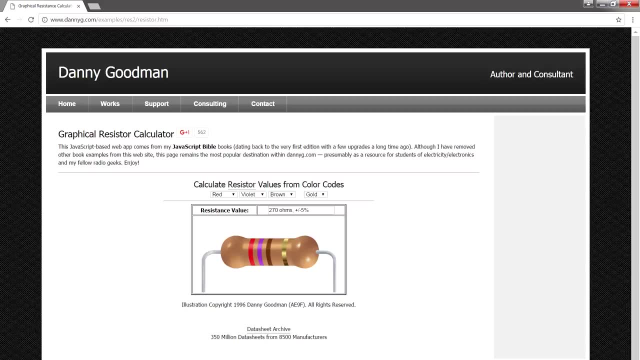 is that there is not satu euchor after zero ohm. So how do you measure resistance between ohm-Re and ohm-Ca in the multimeter? Well, I'm going to show you how to measure resistance between ohm-Ca and ohm-Ca-2. So, in other words, now you know how to measure resistance between ohm-Ca and ohm-Ca. so a multimeter is just some thick layer of resistance that ismoneterized to the insolent atom of energy which causes any resistance, that is an ohm-Ox-DM есте apply to. 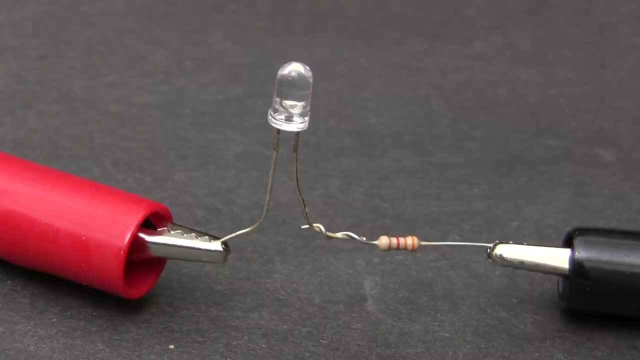 1i-ohm resistance. Ohm-R mild. you need多少 bạn- current that flows in a circuit. Today let's start out with everyone's first simple resistor circuit using a resistor to limit the amount of current going through an LED. Make sure. 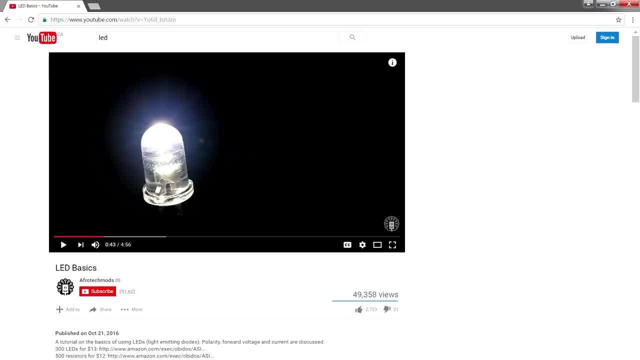 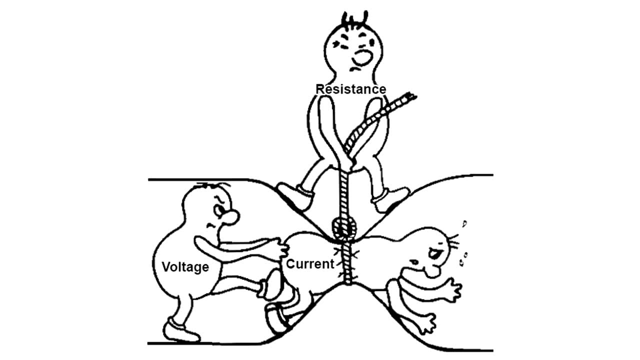 you've already watched my LED tutorial and have bought some resistors and LEDs, which I'm going to link again in the video description section. In order to do the math for this circuit, you need to know about the mathematical relationship between voltage, current and resistance. Here's an old comic that I've always liked: 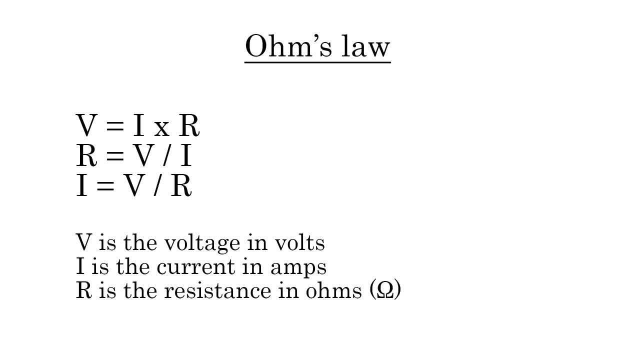 that illustrates this relationship on an intuitive level. More formally, we use this equation Ohm's Law. In textbooks you usually see it written as V equals I times R or voltage equals current times. resistance, If you use a little algebra. 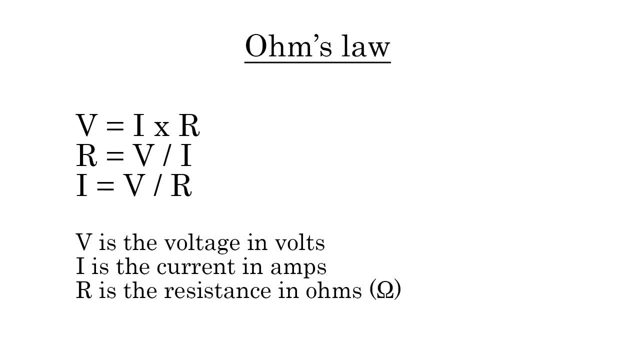 you can rearrange the equation to calculate any of the variables, as long as you know the other two. Although it's important to understand that all these variants of the equation are the exact same thing, our LED circuit is going to be using this version. 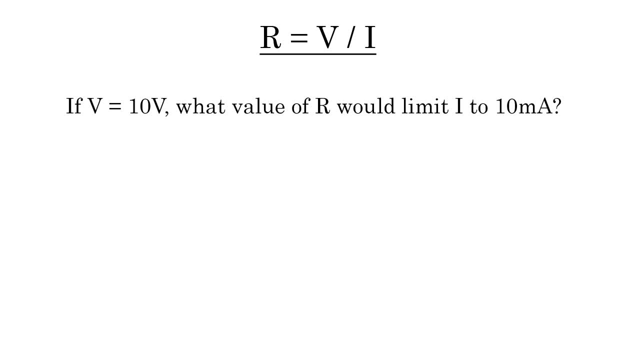 so let's focus on that. Let's say we have a 10V power source and we want to make sure that no more than 10mA flows from it. We can use Ohm's Law to figure out what resistor will accomplish this. 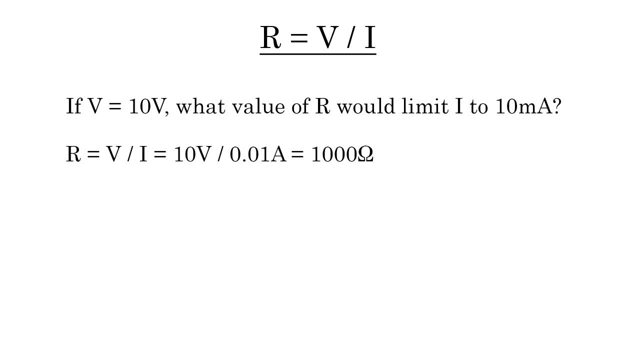 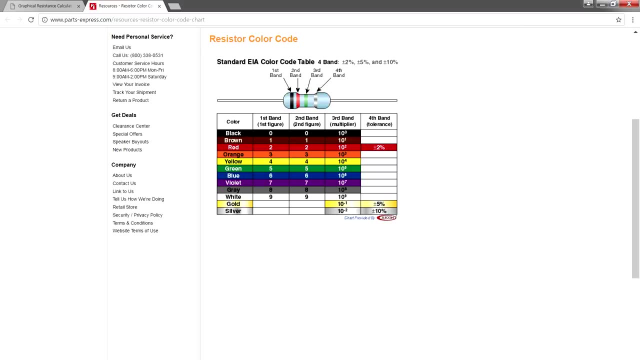 The answer is really simple: Just take the voltage, divide it by the desired current and we get the answer of 1000 Ohms. So now we can either use the resistor color code or a resistor calculator app to figure out what a 1000 Ohm resistor looks like, and it turns out to be brown, black, red, The. 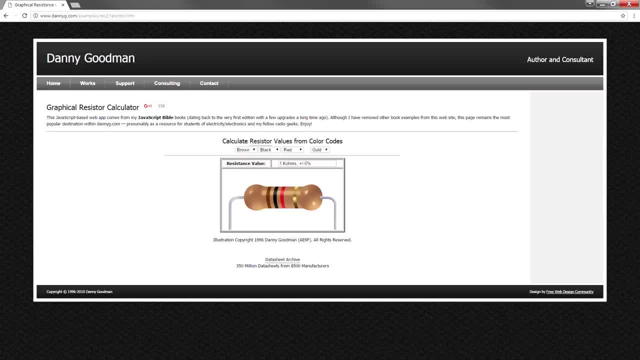 fourth color band: All red. The third color band, all the way on the right, refers to the tolerance of the resistor. A real-world 1000 Ohm resistor might actually have a resistance of 1020 Ohms or 998 Ohms. 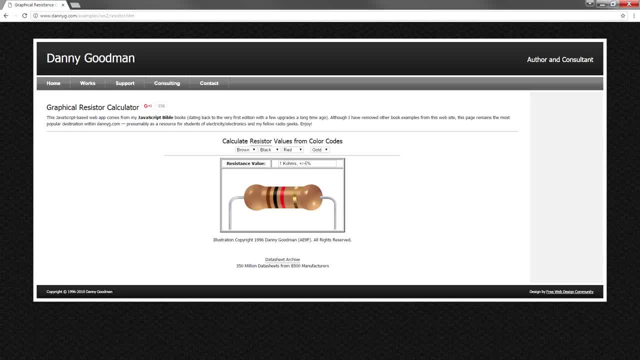 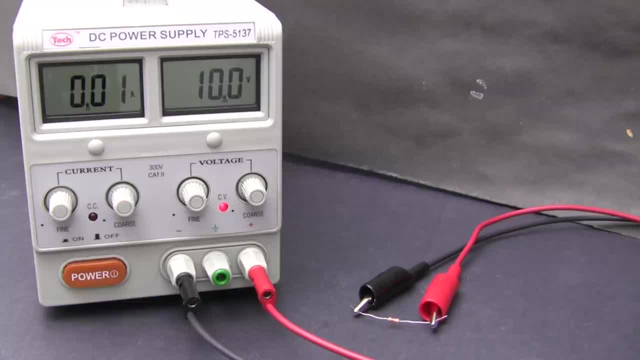 and for most circuits you play with at home, plus or minus 5% will be good enough. So let's double check our math in real life. I've got my power supply set to 10V, it's hooked up to a 1k resistor and, as you'd expect, 10mA is flowing from the power supply. 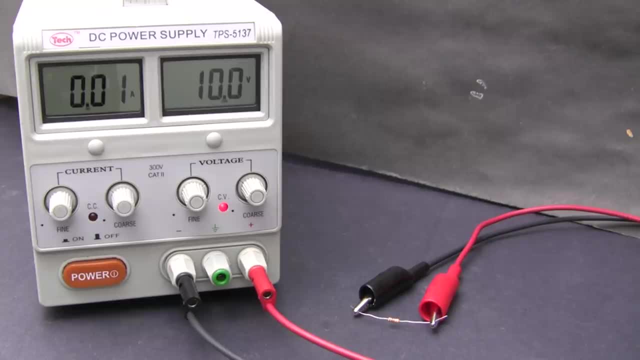 It's also important to know that Ohm's Law is a linear resistance. It's not a linear relationship, meaning that for a fixed resistor value, if you double the voltage, you double the current, Here's 20V going into the same 1000 Ohm resistor and, as you'd expect, the 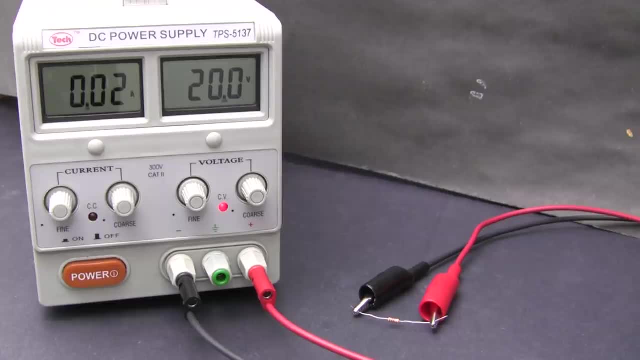 current doubles to 20mA. I want you to understand that only pure, simple resistors obey Ohm's Law. The relationship between voltage and current for most electronics is a lot more complicated than this. In a lot of cases things will work fine right up until their recommended voltage level and 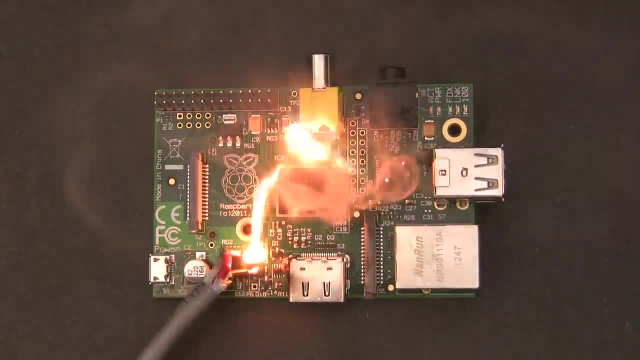 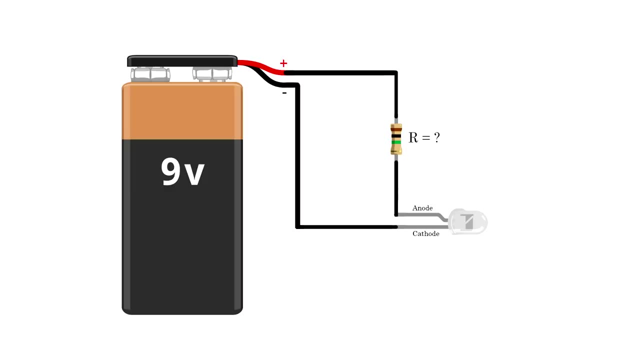 then if you exceed that voltage level, you'll end up with a resistor that's not even as good as the current, But for now, resistors are good enough to help us limit current in a simple LED circuit. Let's start out with a 9V battery, a resistor and an LED connected with the correct polarity. 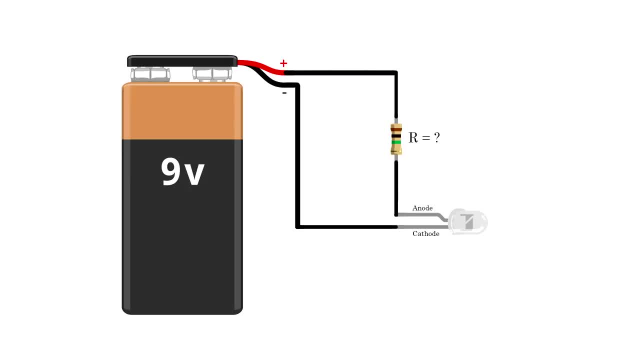 And notice that it doesn't matter which way we connect the resistor. Unlike the LED, polarity doesn't matter for resistors. We want to find out what resistor will let us safely use 9V with this LED. In my previous video about LEDs, we talked about forward voltages. 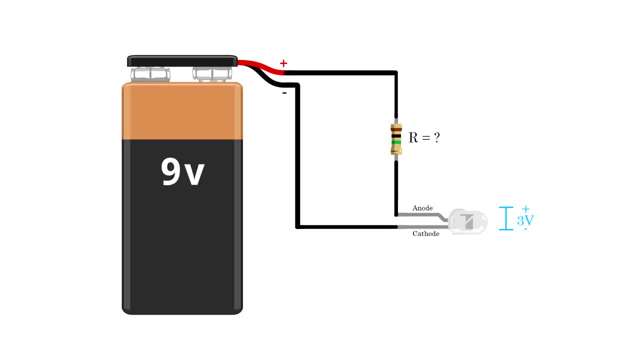 And for this particular white LED, the forward voltage is 3V. That means that when the LED is on, there's going to be a 3V drop across it. So what's the voltage across the resistor? Remember that voltage is all about differences. 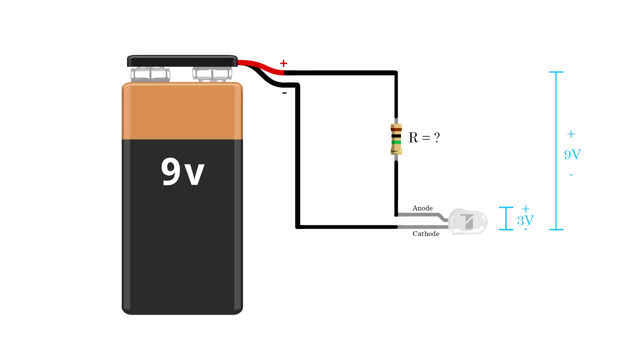 in electrical potential between two points. Our power source is a 9V battery, so we've got 9V between here and here And we've got 3V across the LED. So this must mean that we've got 6V across this resistor, because 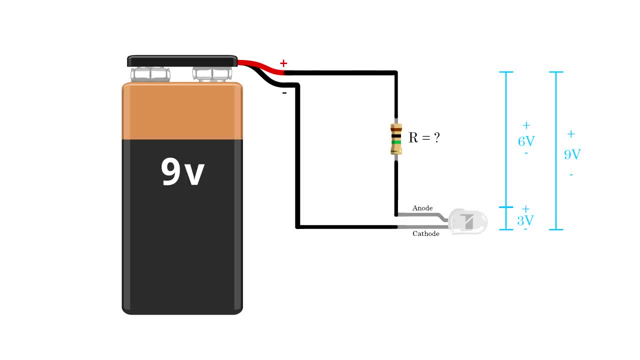 9-3 is 6.. Ok, so we've got our voltage. Now the current in this circuit is going to be whatever we want it to be, But the recommended maximum current for this LED is 20mA, so we're going. 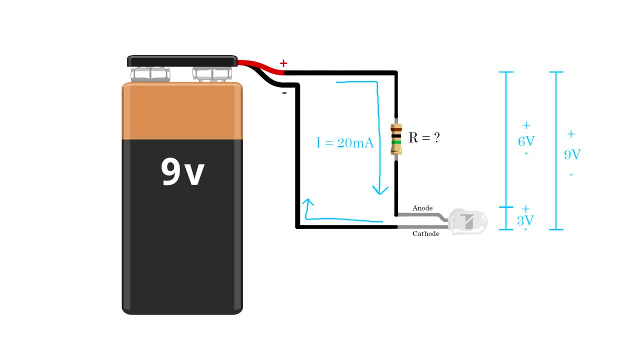 to use that And notice that I'm using conventional current here, which moves from positive to negative. That's what you're going to see in every single electrical engineering situation. but theoretical physics classes might use negative to positive electron flow, So let's apply Ohm's law now. 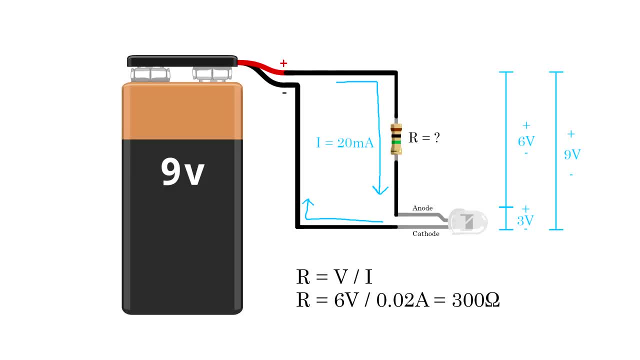 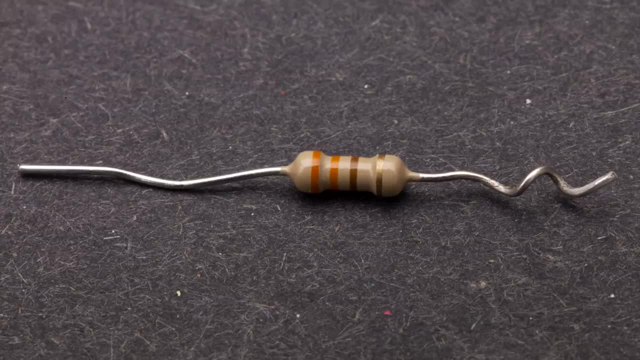 6V divided by 20mA. Now I'm outerly reading so I see a 30 ohm Rel inductance. There's a reason. I'm using that zero, as I'd normally use to VVB, To accelerate my Aahk. I'm holding another switch. 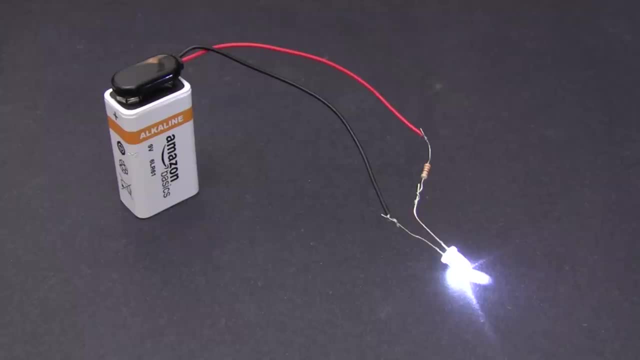 off and the positive charge resistor. Let's see if I can grab that cable. There we go. 9V is correct for the resistor, which means we're going to have equal voltage. If I come back to heat today, the Har Wish här gives us a resistance value of 300 Ohms. Now I don't have a 300 Ohm resistor in my parts collection… but a 330 Ohm resistor'll be good enough if you're messing around with LEDs at home. it doesn't matter if you get the current wrong by 10%. 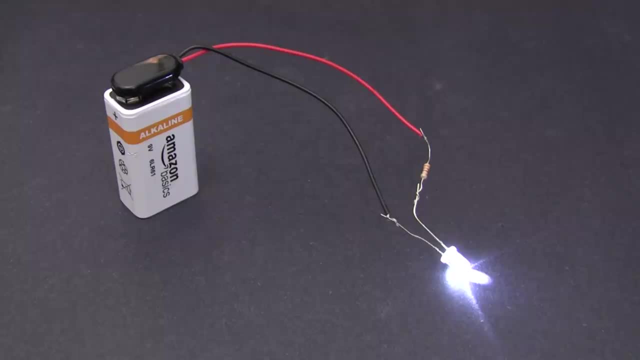 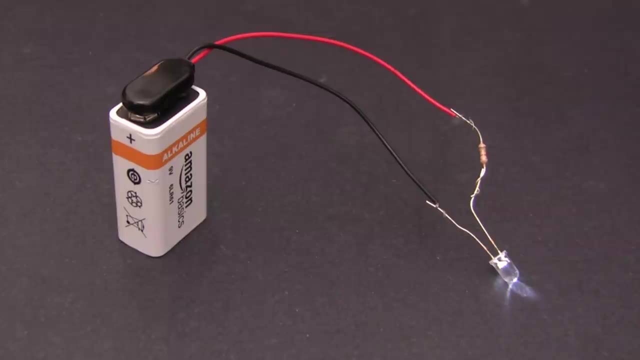 OK, so here I have my 9V battery and a 9V battery clip, 9 volts, roughly 20 milliamps and no exploding LEDs. finally, If we increase the resistance to, let's say, 18 kiloohms, we'll get less current and as 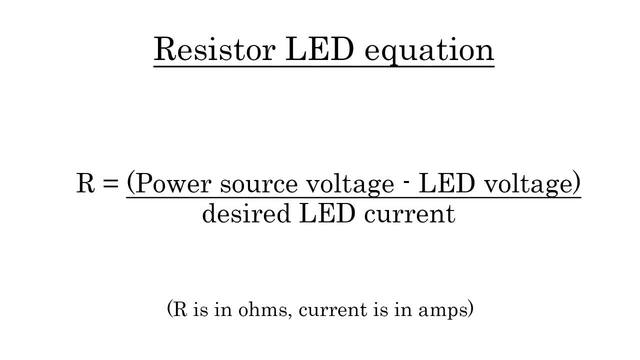 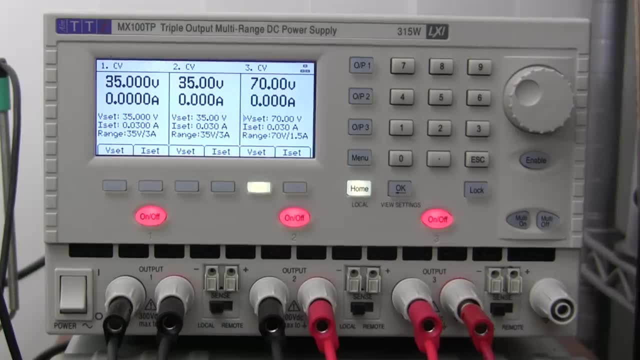 you'd expect, the LED is dimmer In general. this is the equation that you can use to calculate the resistor for a simple LED circuit, But there is a limitation. I've got another power supply here set to give me 140 volts, and that's enough to mess.